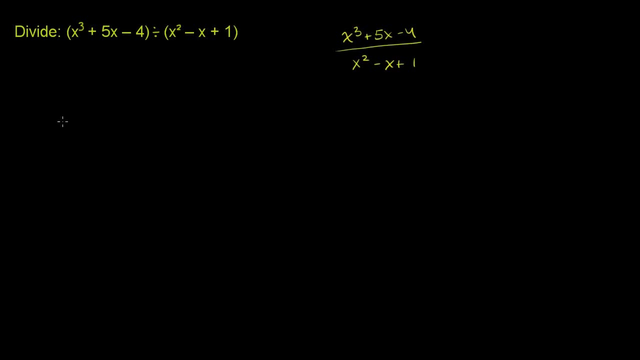 we're going to do algebraic long division is to write it as x squared minus x plus 1 divided into x to the third plus, and actually I'm going to leave some blank space here. We don't have an x squared term here, but I'm going to leave. 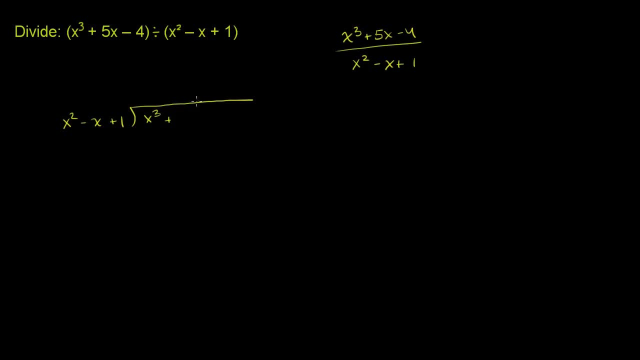 some space for it, just so that we can align everything in the proper place when we actually do this. Let's do the division. So x to the third plus nothing to the x squared power plus 5x minus 4.. So we have a place for the third power, the second power. 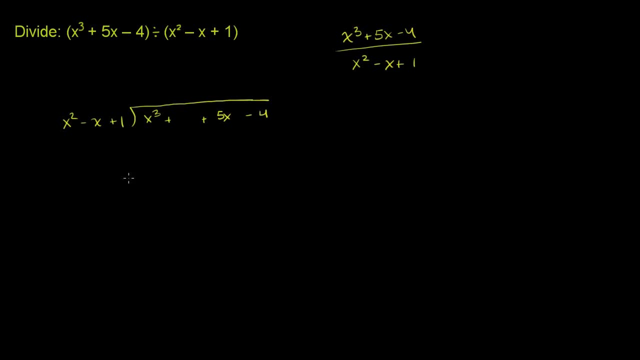 the first power and the zeroth power. So now let's just do a little bit of algebraic long division. Let's look at the highest degree term: x squared goes into x to the third how many times? Well, it goes into it x times. 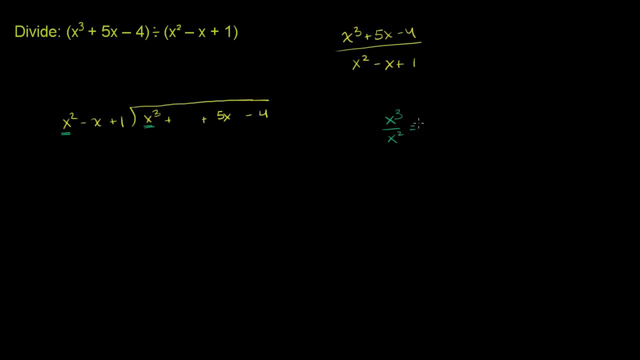 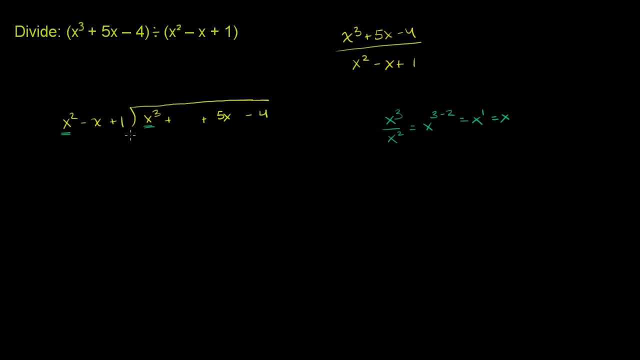 Which is equal to x, to the 1, which is equal to x. So it goes x times. I'll write the x right over here And we multiply x times this entire thing. x times x squared is x to the third. x times negative x is negative x squared. 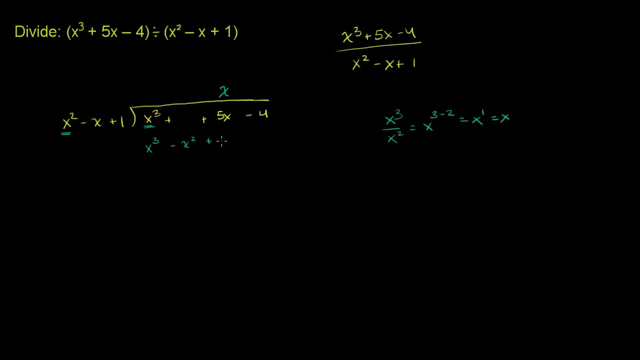 x times 1 is positive x, And now we want to subtract this whole expression from that whole expression, And that's the same thing as adding the opposite or multiplying each of these terms. So we're going to subtract the terms by negative 1 and. 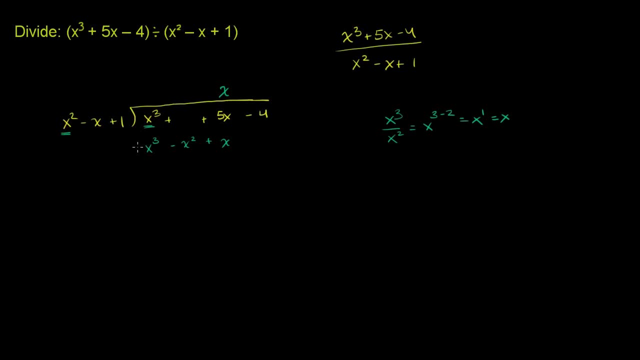 then adding it to these terms. So let's do that. So we have negative x to the third. Negative 1 times negative x squared is positive x squared, And then positive x times negative 1 is negative x. And so let's now add everything. 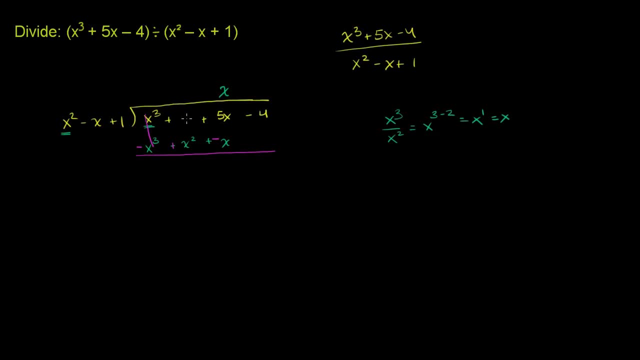 x to the third minus x to the third. those cancel out: 0 plus x squared gives us an x squared. 5x minus x gives us a plus 4x. And then we bring down this minus 4.. We're not adding anything to it. 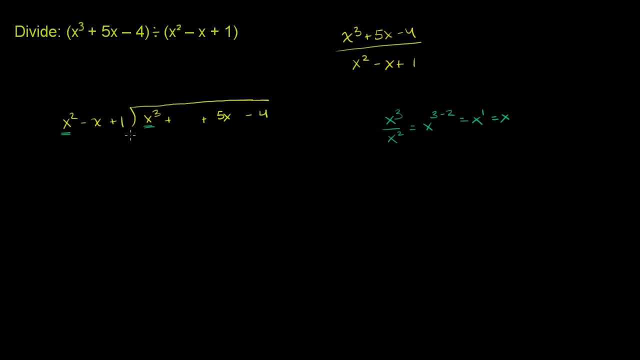 Which is equal to x, to the 1, which is equal to x. So it goes x times. I'll write the x right over here And we multiply x times this entire thing. x times x squared is x to the third. x times negative x is negative x squared. 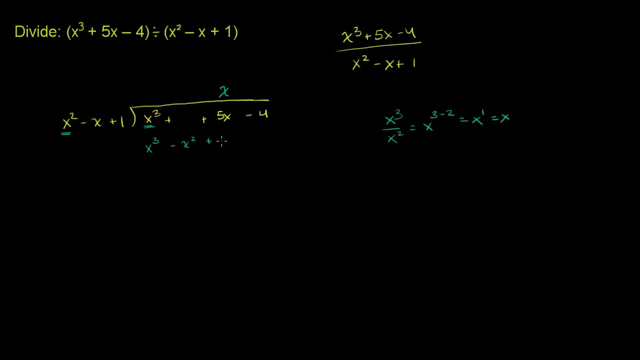 x times 1 is positive x, And now we want to subtract this whole expression from that whole expression, And that's the same thing as adding the opposite or multiplying each of these terms. So we're going to subtract the terms by negative 1 and. 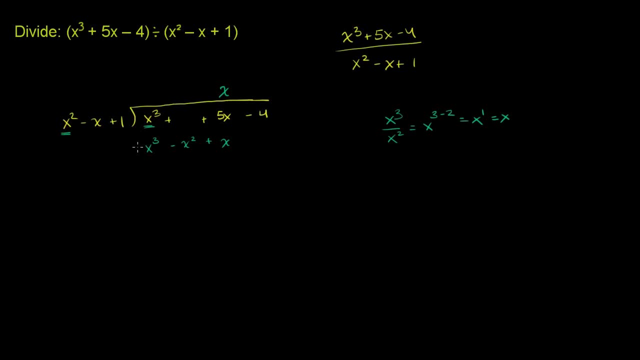 then adding it to these terms. So let's do that. So we have negative x to the third. Negative 1 times negative x squared is positive x squared, And then positive x times negative 1 is negative x. And so let's now add everything. 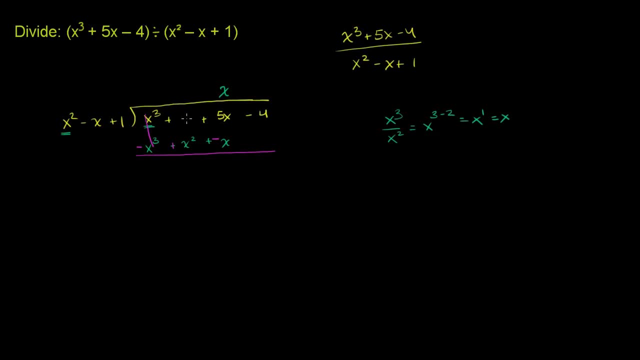 x to the third minus x to the third. those cancel out: 0 plus x squared gives us an x squared. 5x minus x gives us a plus 4x. And then we bring down this minus 4.. We're not adding anything to it. 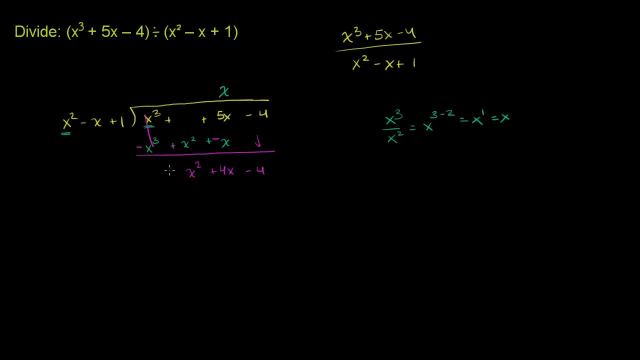 You can view there's a 0 here, So let's bring down the minus 4.. And now let's look at the highest degree terms. x squared goes into x squared- exactly one time It's the same thing. So we put a plus 1.. 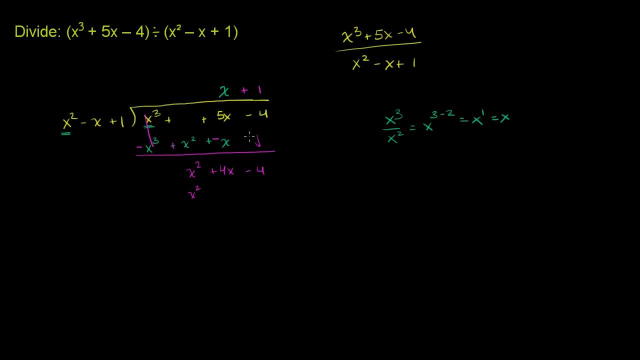 And then you have: 1 times x squared is x squared. 1 times negative x is negative. x 1 times 1 is 1.. And now we want to subtract this from that, Or we want to add the opposite. To add the opposite. 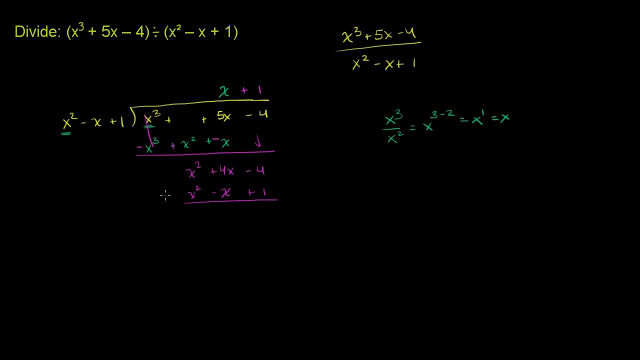 We can just multiply each of these terms by negative 1.. x squared becomes negative, x squared Negative. x times negative 1 is positive x. And then positive 1 times negative 1 is negative 1.. Now let's do the addition. 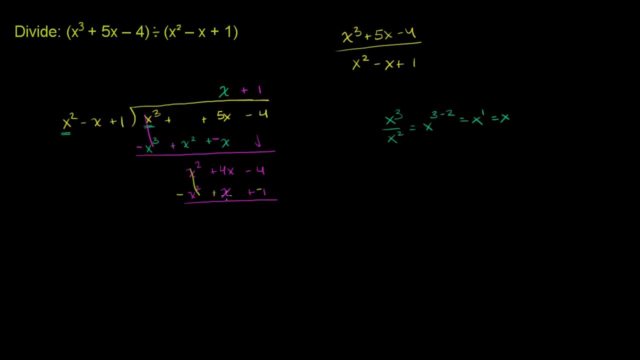 x squared minus x squared, they cancel out. 4x plus x is 5x, And then we have negative 4 minus 1 is negative 5.. Now you might be tempted to keep dividing, But you can't anymore. 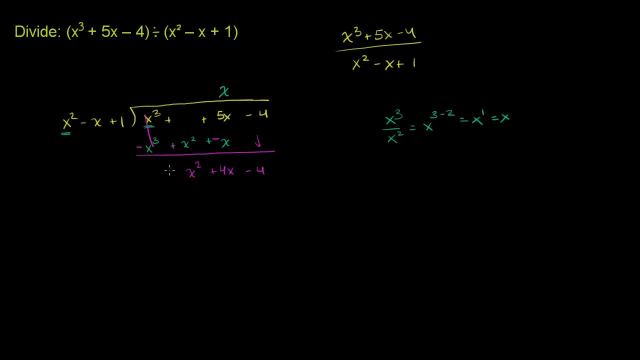 You can view there's a 0 here, So let's bring down the minus 4.. And now let's look at the highest degree terms. x squared goes into x squared- exactly one time It's the same thing. So we put a plus 1.. 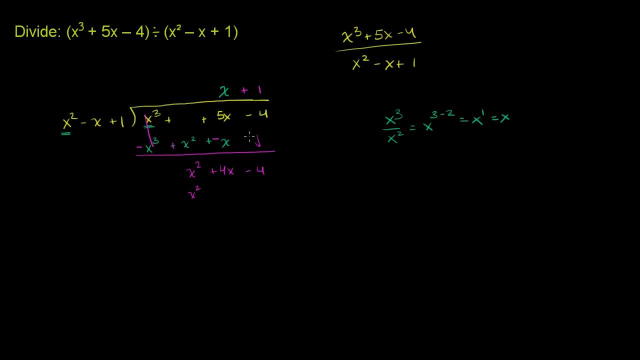 And then you have: 1 times x squared is x squared. 1 times negative x is negative. x 1 times 1 is 1.. And now we want to subtract this from that, Or we want to add the opposite. To add the opposite. 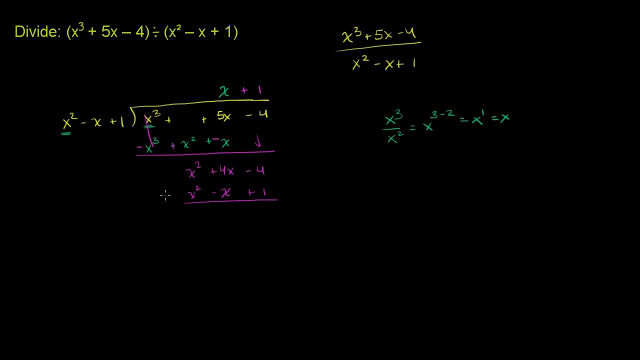 We can just multiply each of these terms by negative 1.. x squared becomes negative, x squared Negative. x times negative 1 is positive x. And then positive 1 times negative 1 is negative 1.. Now let's do the addition. 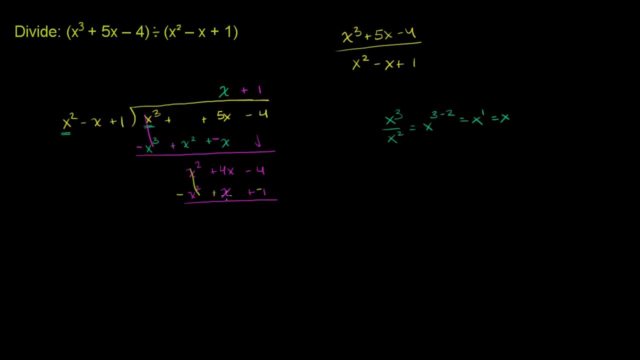 x squared minus x squared, they cancel out. 4x plus x is 5x, And then we have negative 4 minus 1 is negative 5.. Now you might be tempted to keep dividing, But you can't anymore. 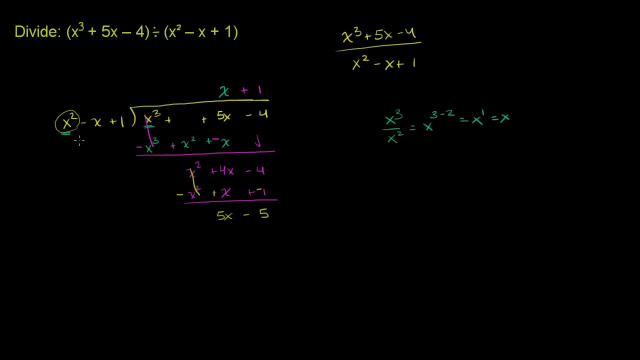 This term right here. the highest degree term here is now higher than the highest degree term that you're going to try to divide into, So we have a remainder. So the answer to this is this: expression right over here is equal to x plus 1.. 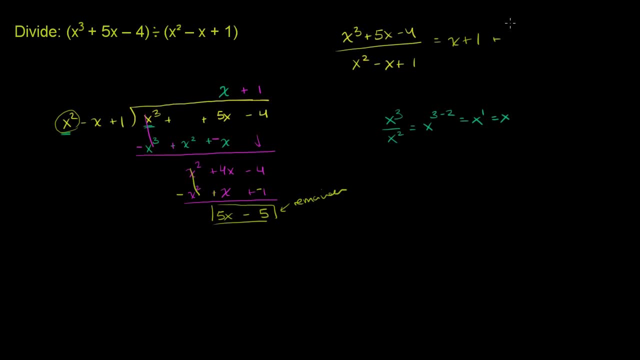 This: x plus 1 plus the remainder, plus 5x squared 5x minus 5.. Whatever, the remainder is divided by x squared minus x plus 1.. If this was divisible, we could keep dividing, But we're saying it's not. 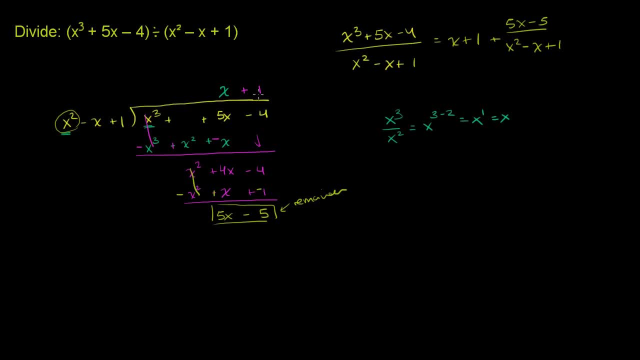 It's now a lower degree than this down here. So we could say: it's x plus 1 plus whatever. this remainder is divided by this thing over here. So our answer- I'm going to write it one more time- It's x plus 1 plus 5x minus 5.. 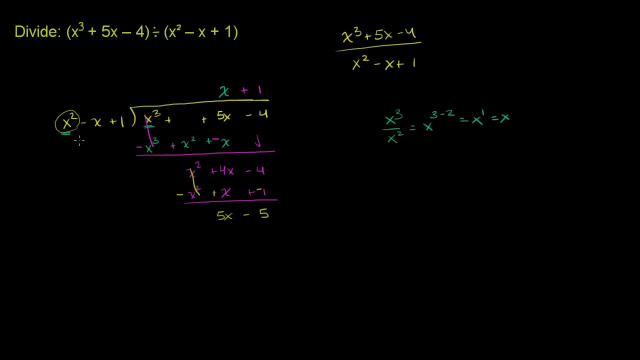 This term right here. the highest degree term here is now higher than the highest degree term that you're going to try to divide into, So we have a remainder. So the answer to this is this: expression right over here is equal to x plus 1.. 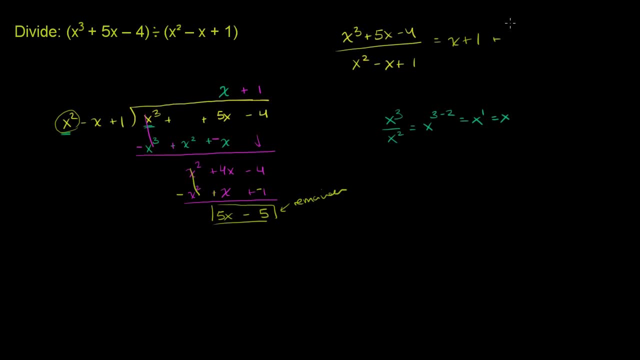 This: x plus 1 plus the remainder, plus 5x squared 5x minus 5.. Whatever, the remainder is divided by x squared minus x plus 1.. If this was divisible, we could keep dividing, But we're saying it's not. 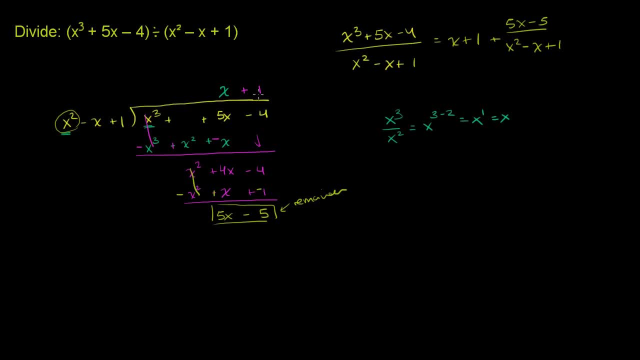 It's now a lower degree than this down here. So we could say: it's x plus 1 plus whatever. this remainder is divided by this thing over here. So our answer- I'm going to write it one more time- It's x plus 1 plus 5x minus 5.. 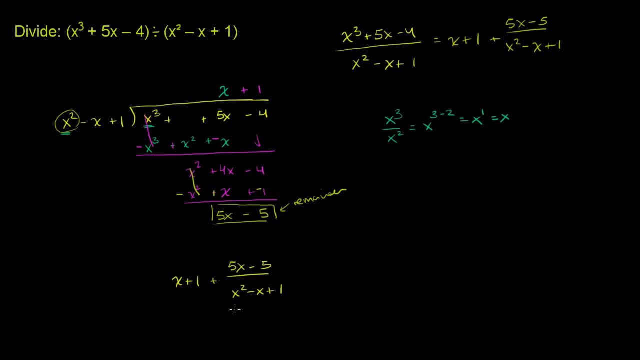 5 over x, squared minus x plus 1.. And we can check that this works If we take this thing over here and we multiply it by this thing over here, we should get the x to the third plus 5x minus 4.. 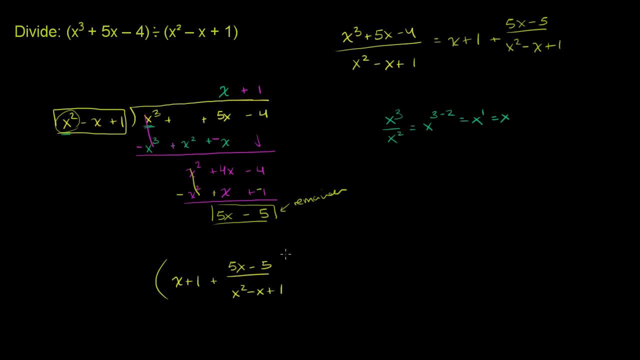 So let's do that, Let's multiply this thing, Let's multiply it by x squared minus x plus 1.. And to do that, let's just distribute this whole trinomial: times, each of these terms, Times, each Times, each of these terms. 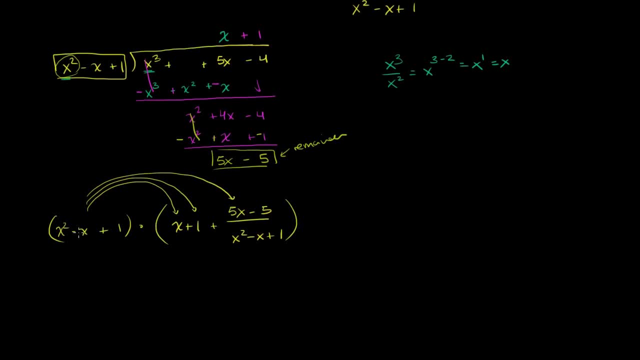 When we do the first term, we have x squared minus x, plus 1 times x. So that's going to be x times x squared, which is x to the third, x times negative x, which is negative, x squared x times 1, which is plus x. 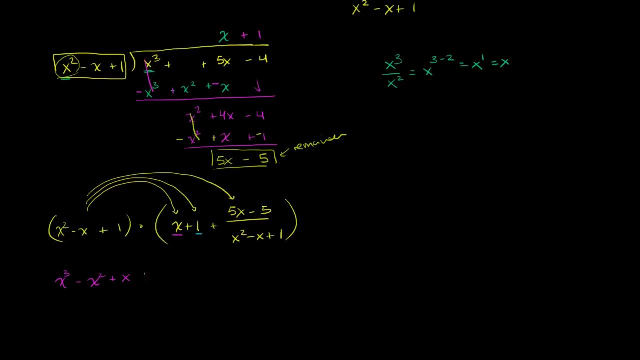 Then we can multiply this whole thing times 1.. So it's going to be plus x squared minus x plus 1.. I'm just multiplying all of these times 1.. And then we can multiply this whole thing times this thing. Now, this is the same as the denominator here. 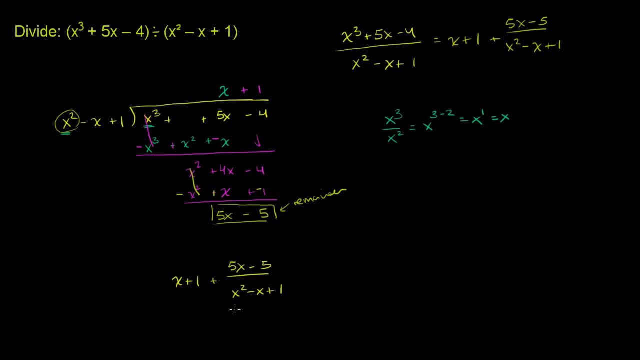 5 over x, squared minus x plus 1.. And we can check that this works If we take this thing over here and we multiply it by this thing over here, we should get the x to the third plus 5x minus 4.. 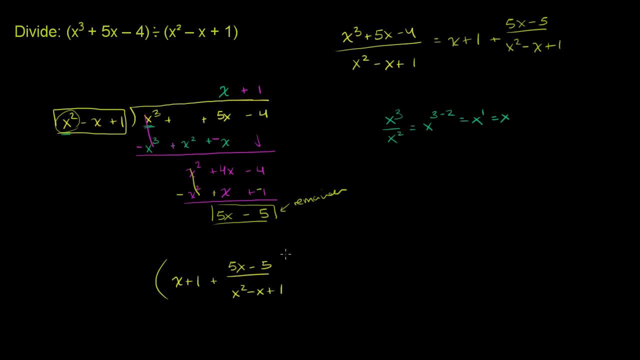 So let's do that, Let's multiply this thing, Let's multiply it by x squared minus x plus 1.. And to do that, let's just distribute this whole trinomial: times, each of these terms, Times, each Times, each of these terms. 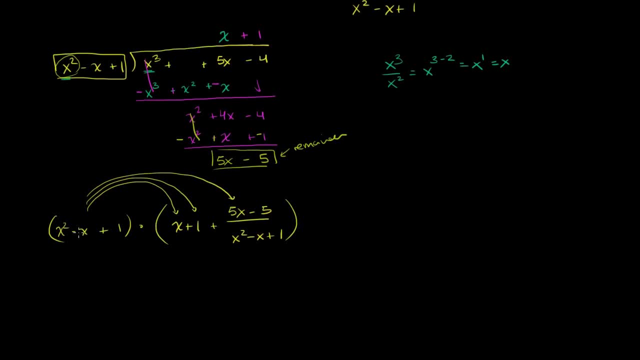 When we do the first term, we have x squared minus x, plus 1 times x. So that's going to be x times x squared, which is x to the third, x times negative x, which is negative, x squared x times 1, which is plus x. 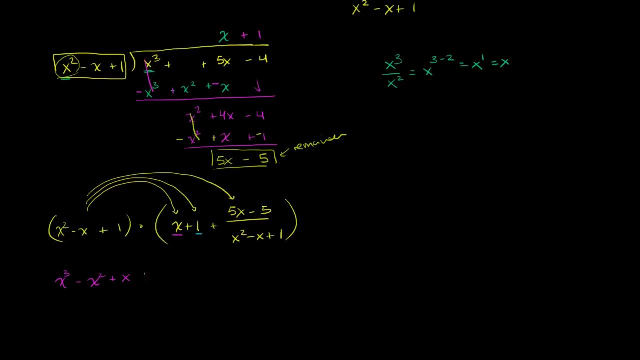 Then we can multiply this whole thing times 1.. So it's going to be plus x squared minus x plus 1.. I'm just multiplying all of these times 1.. And then we can multiply this whole thing times this thing. Now, this is the same as the denominator here. 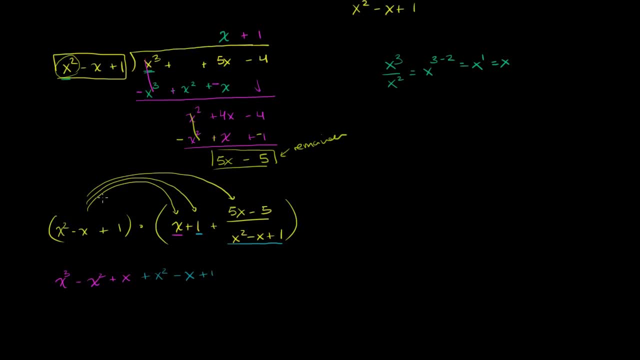 so it'll cancel out. This will cancel with that, and we're just going to be left with the numerator over here. So plus 5x, minus 5.. And now we can try to simplify it. We only have one third degree term, the x to the third. 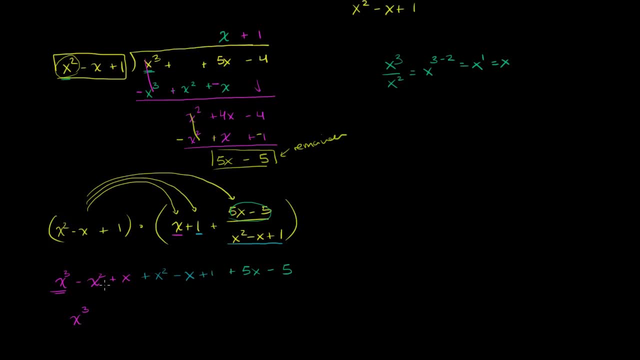 So we have x to the third here, Second degree terms, we have a negative x squared and then we also have a positive x squared, So they cancel out with each other. First degree terms. Let's see We have a positive x and a negative x. 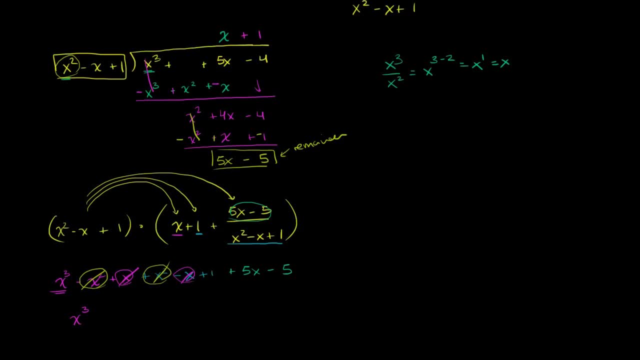 Those cancel out with each other. So we're just going to have that 5x over here. So we're just going to have this 5x. So then we have plus 5x And then we have the 0th degree terms or the constant terms. 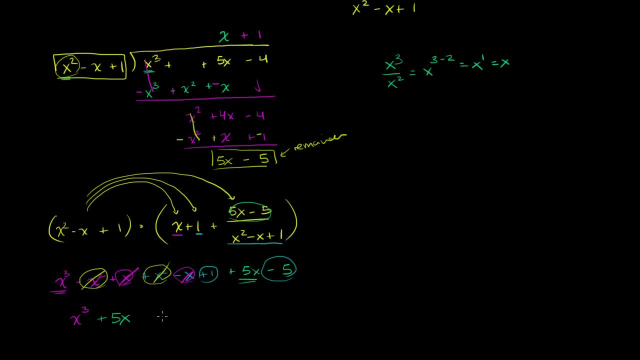 We have a positive 1 and a negative 5. Add them together, you get negative 4. So you get x to the third plus 5x, minus 4, which is exactly what we had over here. 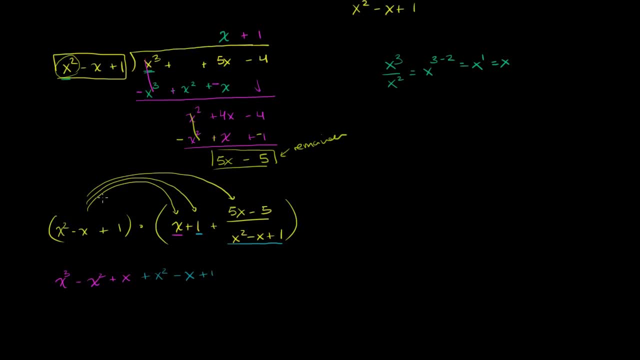 so it'll cancel out. This will cancel with that, and we're just going to be left with the numerator over here. So plus 5x, minus 5.. And now we can try to simplify it. We only have one third degree term, the x to the third. 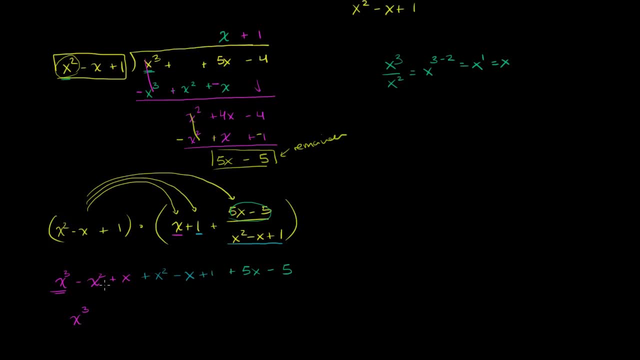 So we have x to the third here, Second degree terms, We have a negative x squared and then we also have a positive x squared, So they cancel out with each other. First degree terms. Let's see We have a positive x and a negative x. 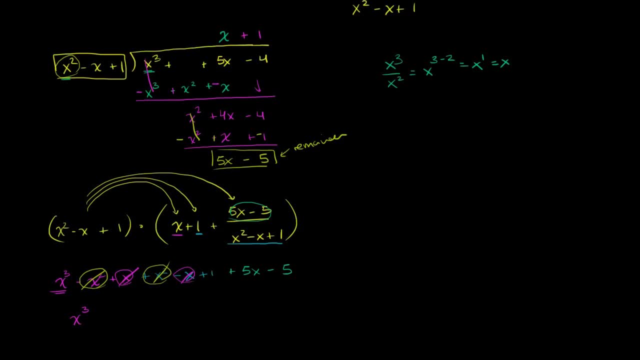 Those cancel out with each other. So we're just going to have that 5x over here. So we're just going to have this 5x. So then we have plus 5x And then we have the 0th degree terms or the constant terms. 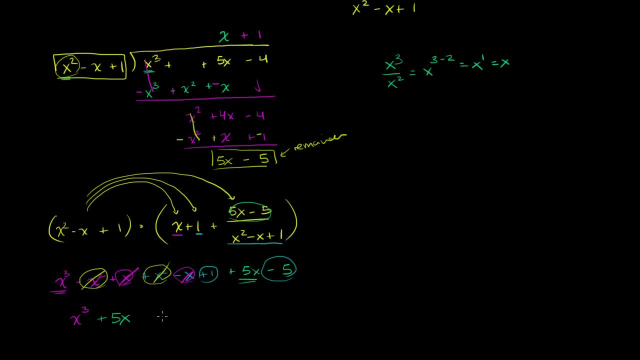 We have a positive 1 and a negative 5. Add them together, you get negative 4. So you get x to the third plus 5x, minus 4, which is exactly what we had over here. 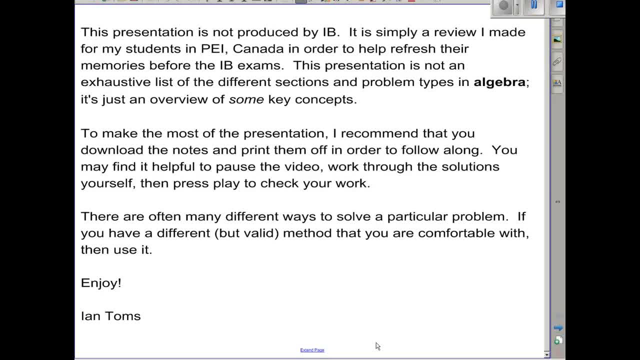 Hi folks, welcome to the algebra review for the Math SL exams. Basically, in this section you'll be looking at arithmetic sequences and series, geometric sequences and series, logarithms and binomial expansions. This is not endorsed or produced by the IB. it's just a little review that I made for my students in PEI Canada. 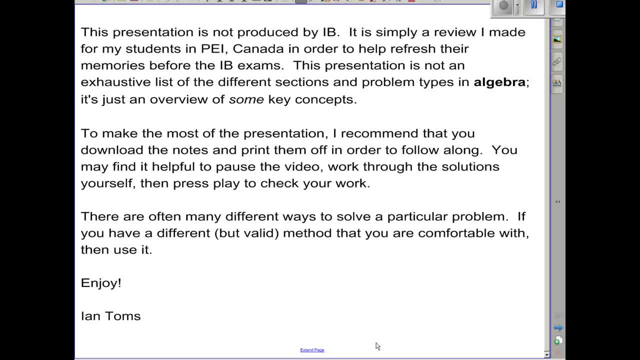 You can print off the notes. just follow the link that's below and you might find the most useful thing to be to print off those notes, work through the solutions and then use the presentation to check your work. There are often a lot of different ways to solve a particular problem, so if you have a different way that you've been taught perfect, Please use that. 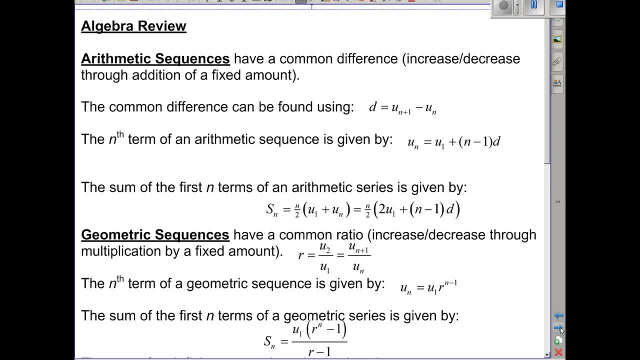 Okay, arithmetic sequences are sequences that have a common difference, which means they go up or down by a fixed amount through addition. So we're going to look at arithmetic sequences. Okay, arithmetic sequences are sequences that have a common difference, which means they go up or down by a fixed amount through addition. 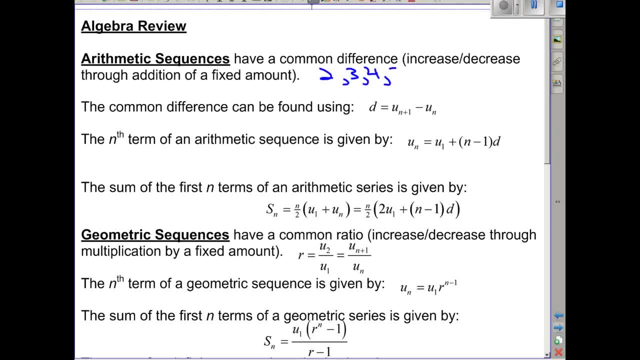 So the sequence 2,, 3,, 4, 5 would be a pretty straightforward arithmetic sequence. It's got a common difference of 1.. If I wrote it as 5,, 4,, 3,, 2, etc. then you're looking at still an arithmetic sequence, but here the difference has changed.